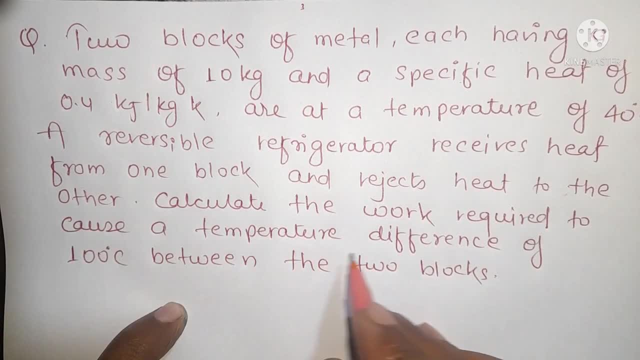 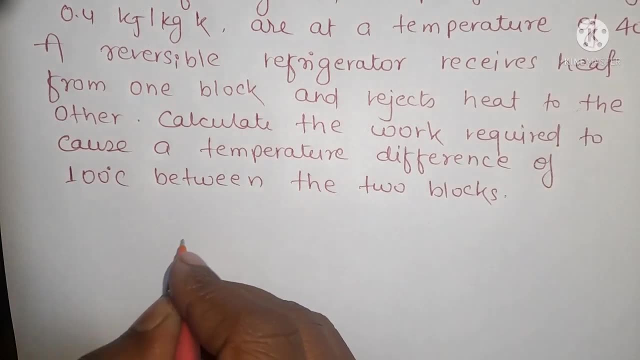 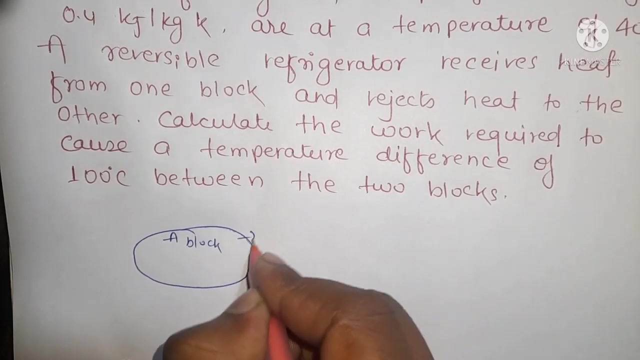 Calculate the work required to cause a temperature difference of 100°C between the two blocks? Question says that we have two blocks and both the blocks whose mass, specific heat and temperature are the same. Suppose we have a block whose mass is 10 kg. 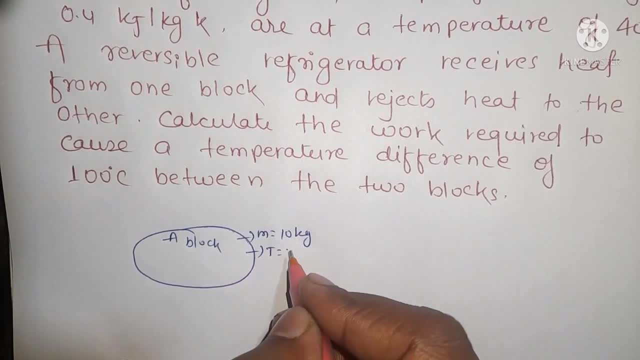 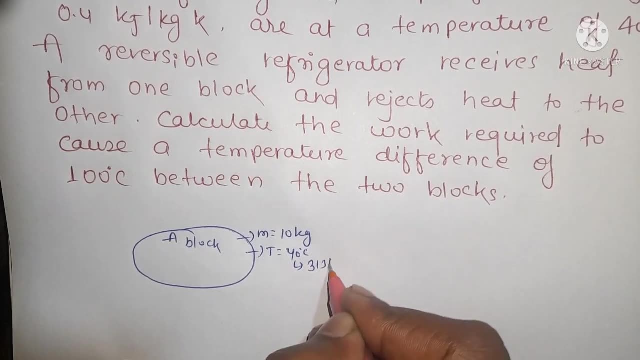 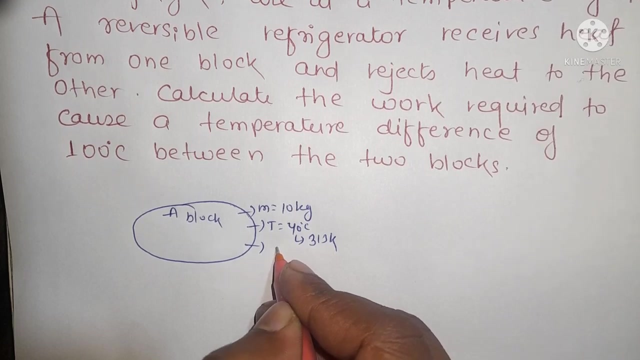 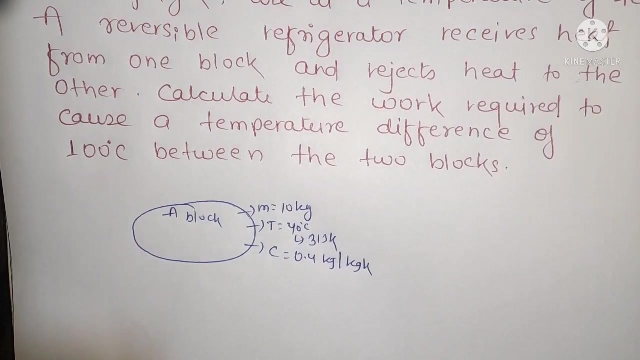 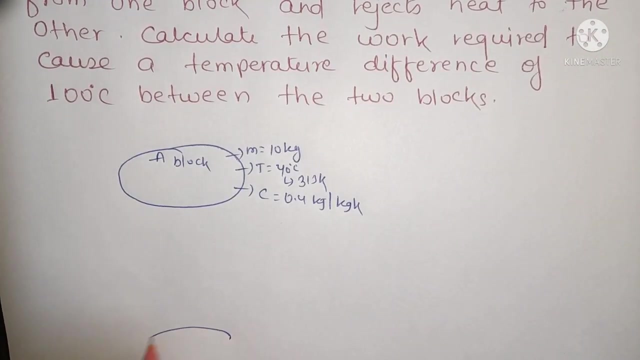 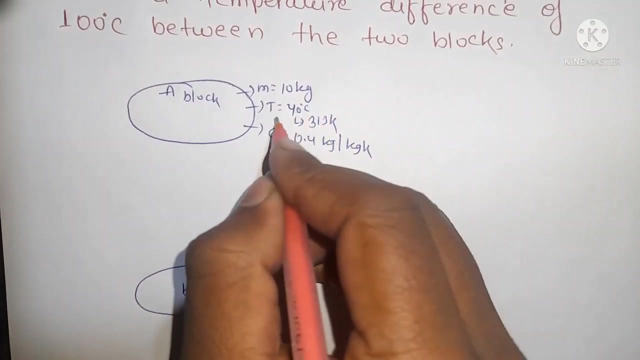 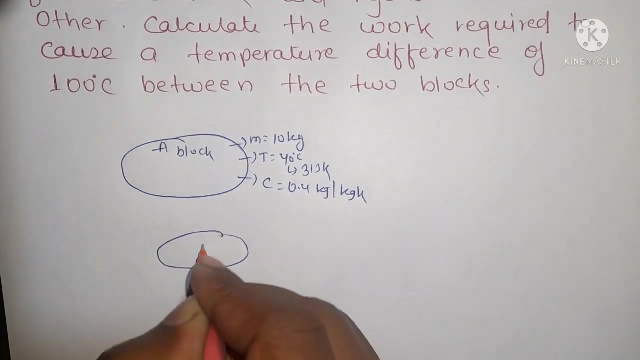 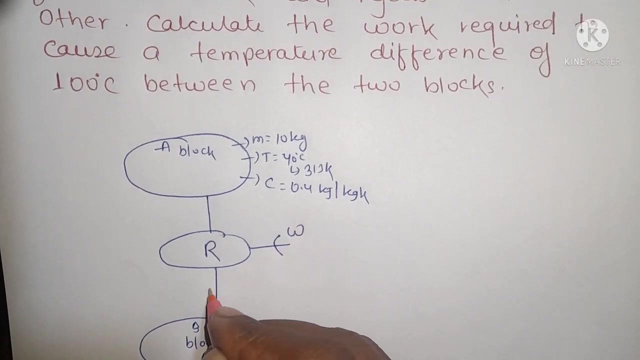 And its temperature is 40°C. When we add 273 K it will be 313 K And its specific heat is 0.4 kJ per kgK. That's it. And the second job is: The block given here has the same mass, temperature and specific heat and a reversible refrigerator is installed between the two blocks and when you input the work in the refrigerator it will take the heat from the lower temperature and input it in the higher temperature. 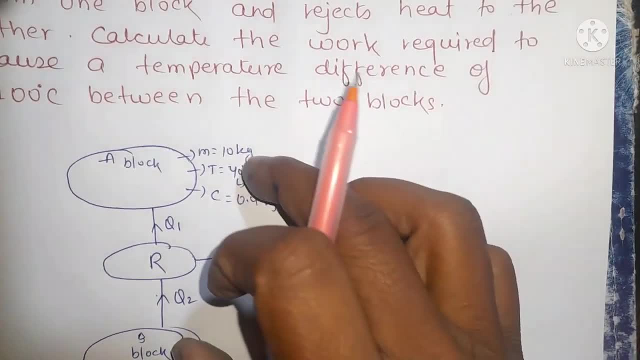 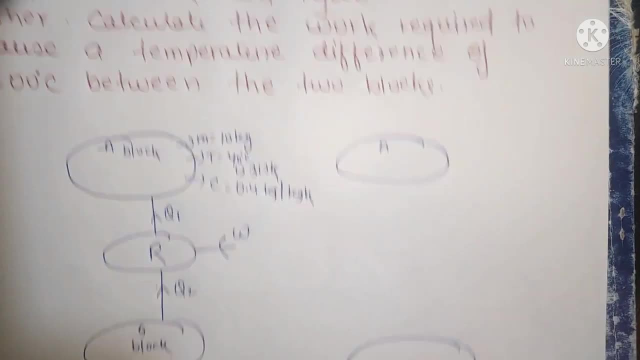 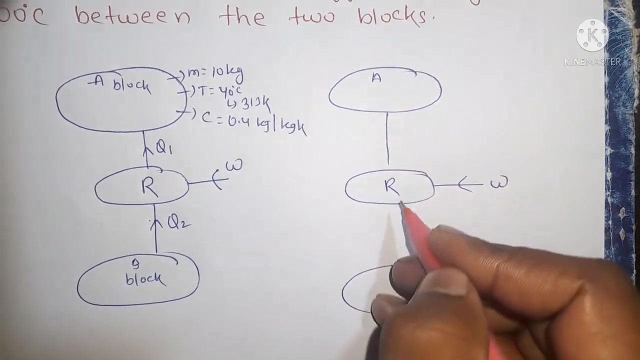 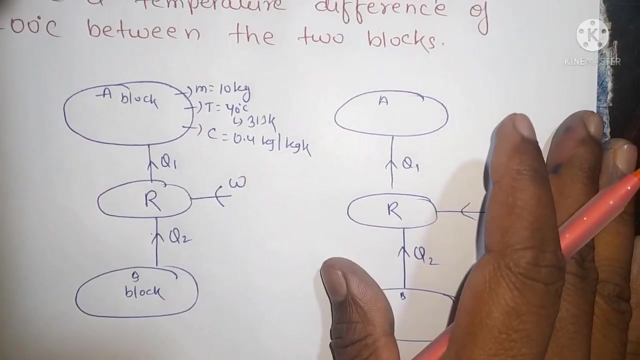 If the temperature of the two blocks is the same, then the block given here is a block and the block given here is b block and the refrigerator is set up between them and the work is being input. And the question is how much work is required. 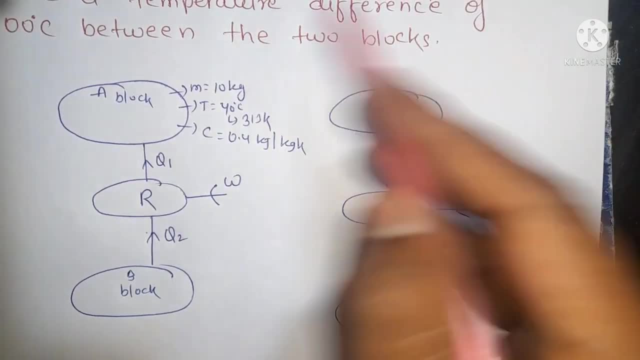 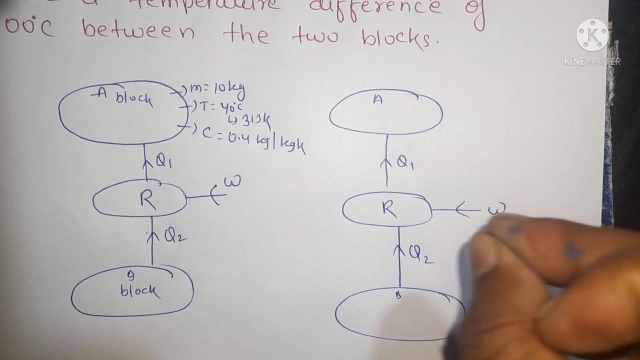 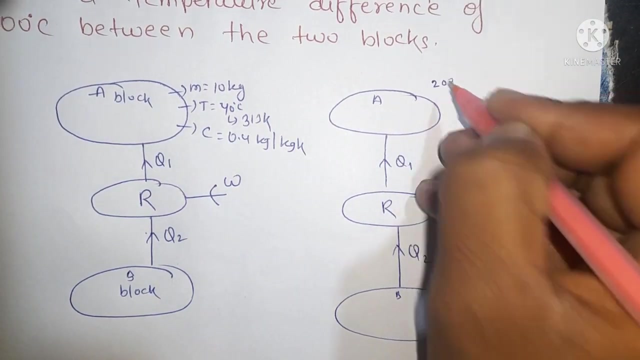 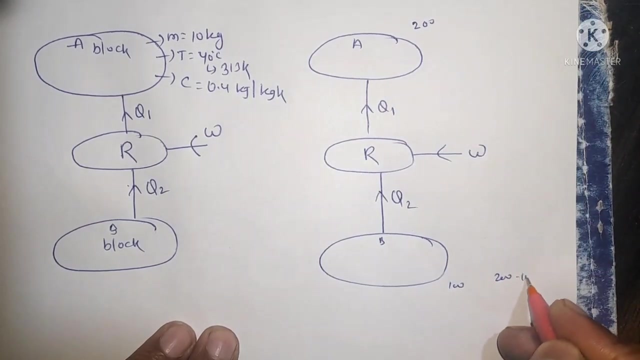 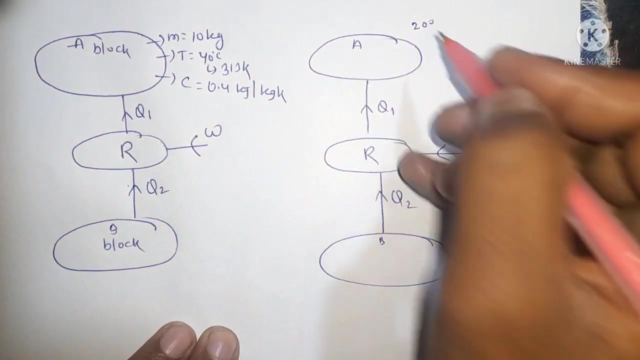 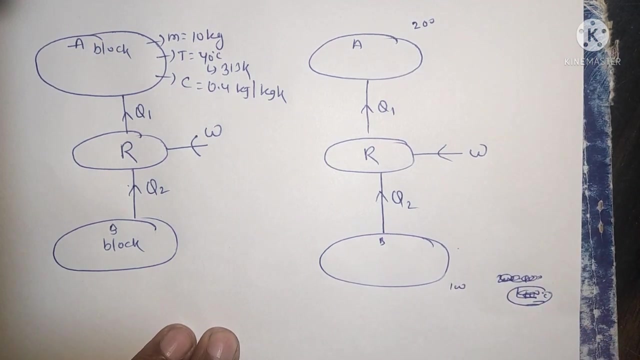 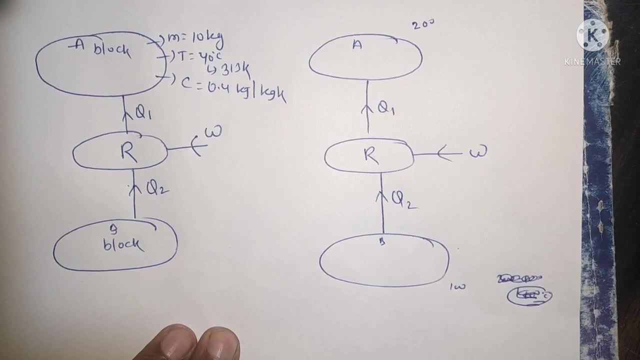 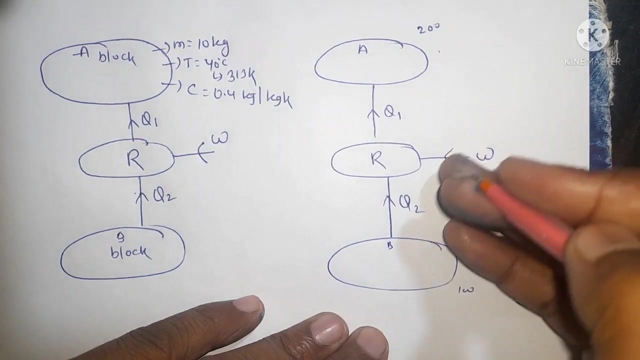 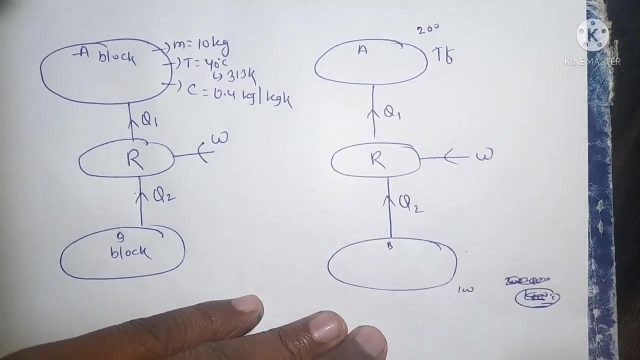 so to keep 100 degree Celsius temperature difference? how much amount of work you have to input in this? I have to find out the value. suppose this body is taking out any amount of heat, so its temperature is increasing. earlier it was 40 degree Celsius and now its Tf is increasing. 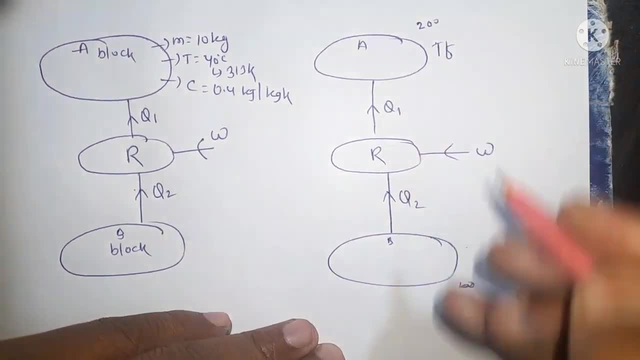 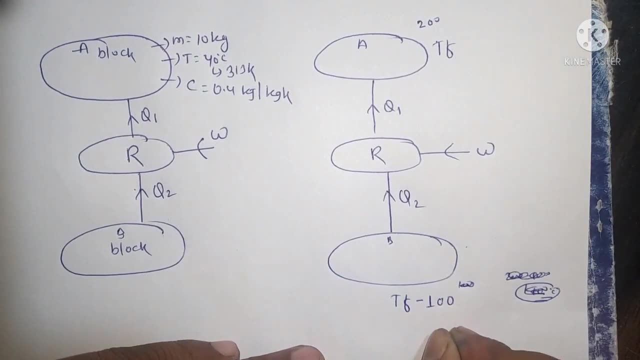 and its temperature is Tf. so we have to do Tf minus 100 degree Celsius. why we have to do it? because we will reduce 100 degree Celsius from Tf, so we will subtract the final minus initial. then our 100 degree Celsius temperature difference will be saved. 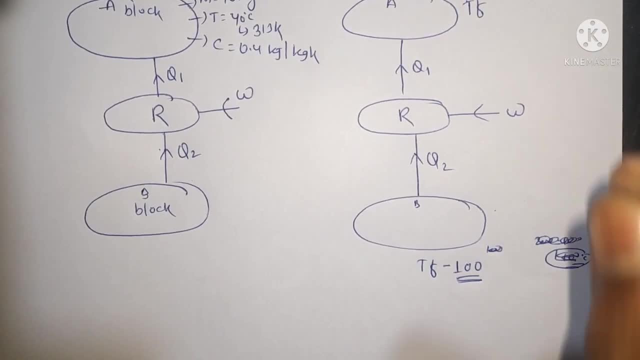 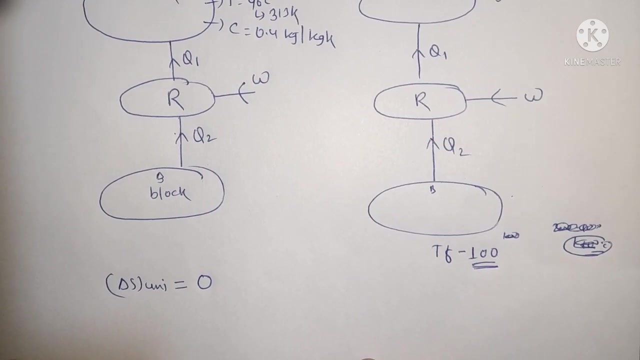 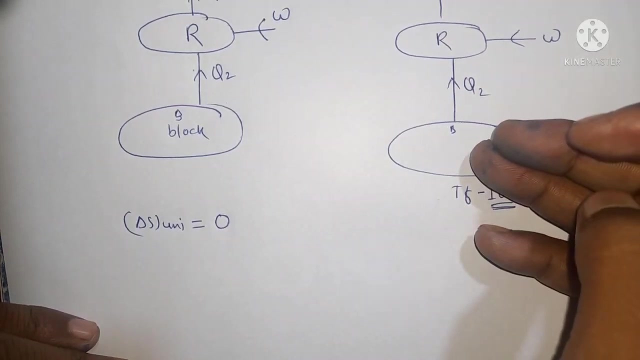 so now I have to do work. see our process. this cycle of refrigerator comes for reversible cycle. so reversible change, entropy of universe change. entropy of the universe for reversible cycle is zero. now our universe is not going in A system and B system, but it is going in A from B. 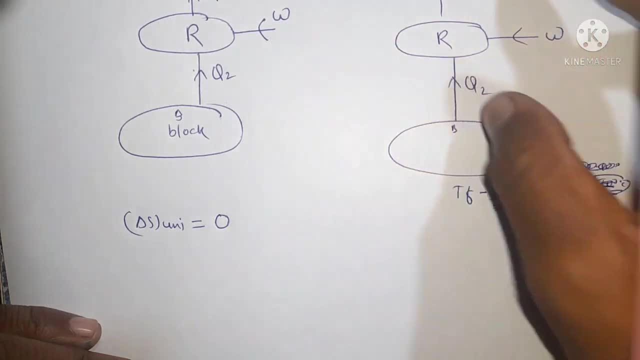 from B to A means your system is saved here and doesn't hit anywhere at all at surrendering point of residual heat. it is going in B, then going in A. from B to A means your system is safe here and there is no heat at surrendering point of residual heat. 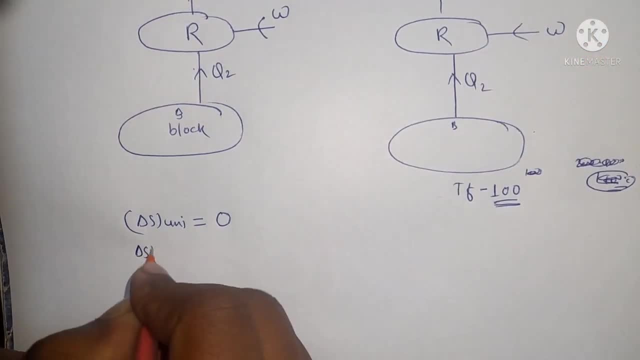 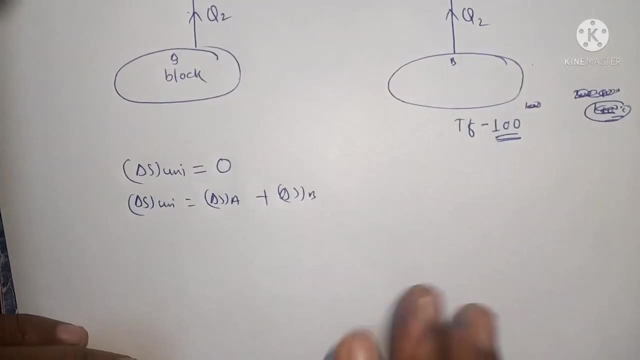 change in entropy is 0. so how is the system made? the universe is made entropy change of A plus entropy change of B. ok, so equal to 0. ok, so your entropy change will be dq by T. and where is its temperature going? its temperature is going. 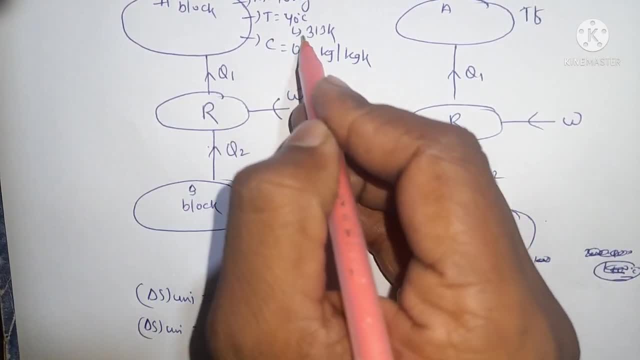 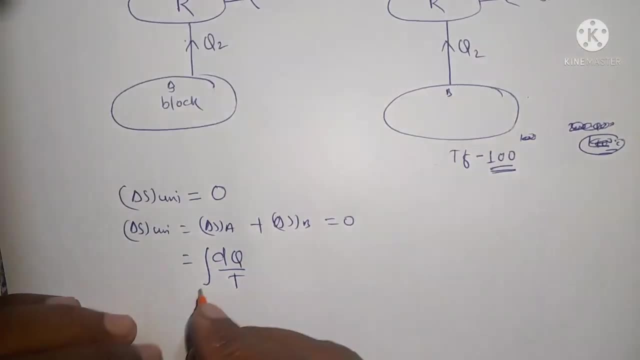 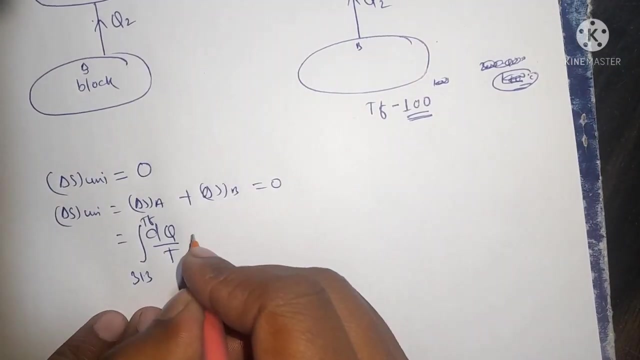 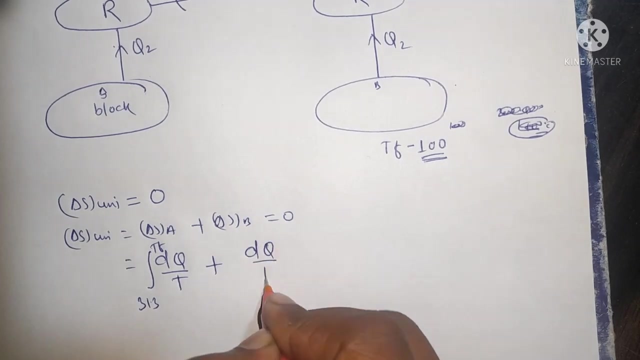 the body of A, its temperature is going, your temperature is going 313, 313, 313, 313 to Tf, 313 to Tf. ok, and your body, or block from which we are getting heat, its temperature was earlier. its formula was dq by T, it was 313 earlier. 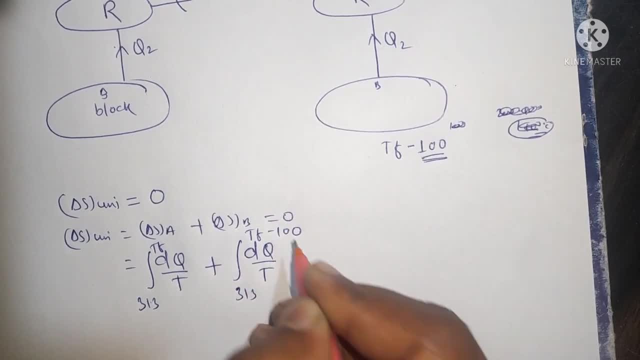 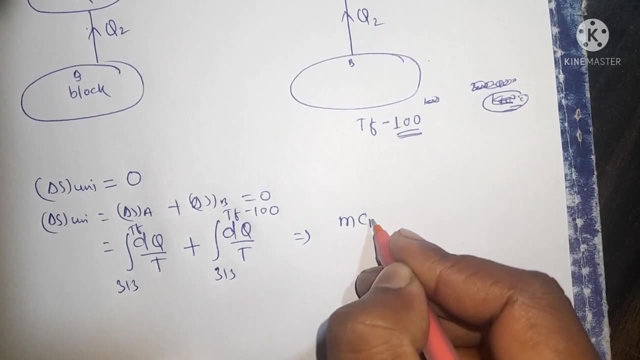 but now its temperature is Tf minus 100 degree Celsius. ok, so what is dq formula? dq formula is mc into dT by T, dT is heat mc dT and dT is dT is 313 to Tf, 313 to Tf, plus mc dT by T. 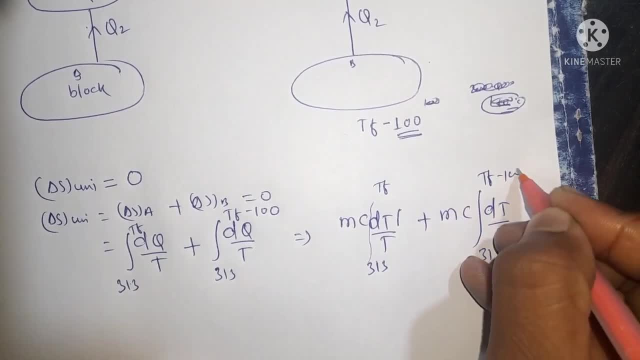 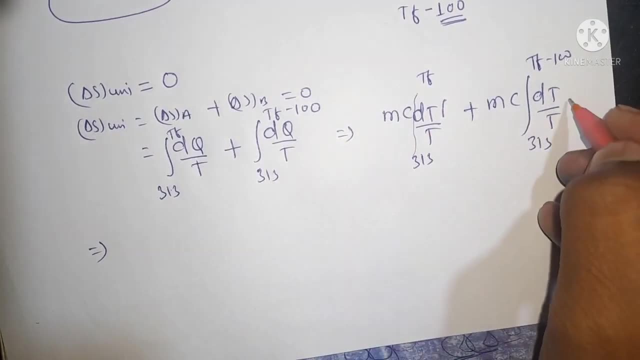 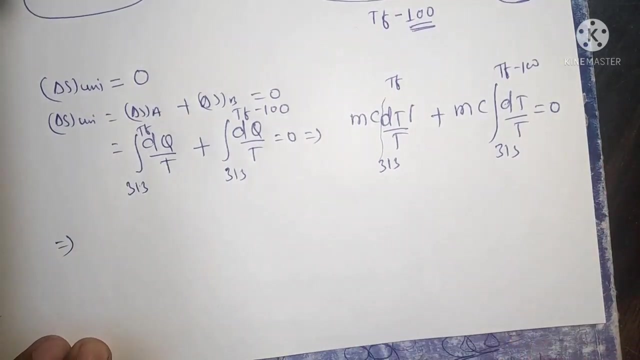 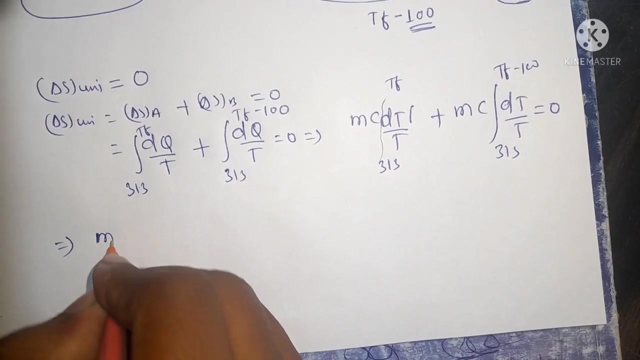 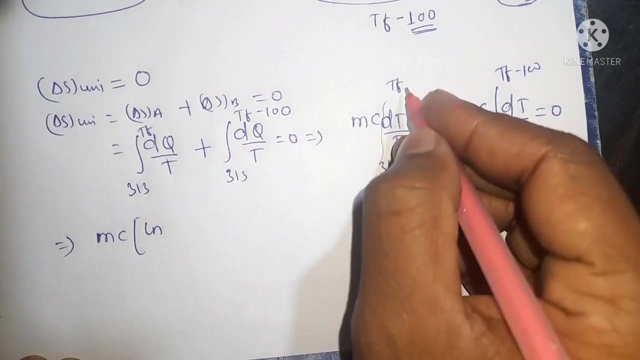 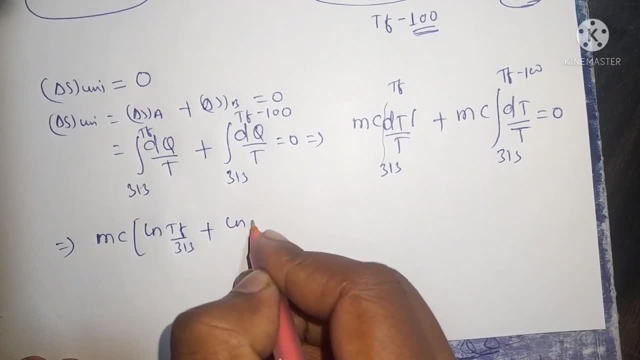 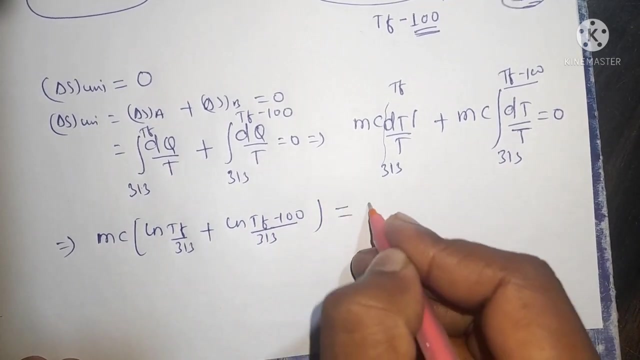 you will integrate t of this. also l and t will come and you will put value of t. so your final initial, from where it is going from 313 to tf minus 100 into zero, when you will bring mcp here, then your zero will be l and t, tf by 313. 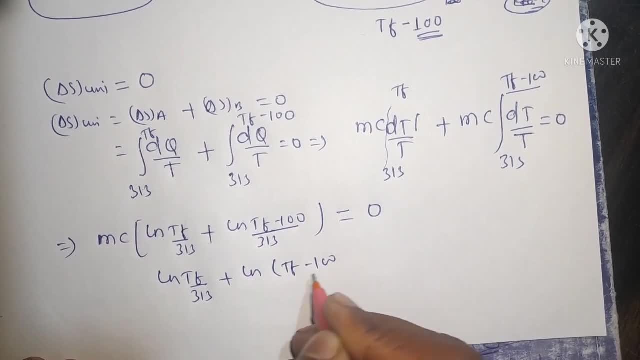 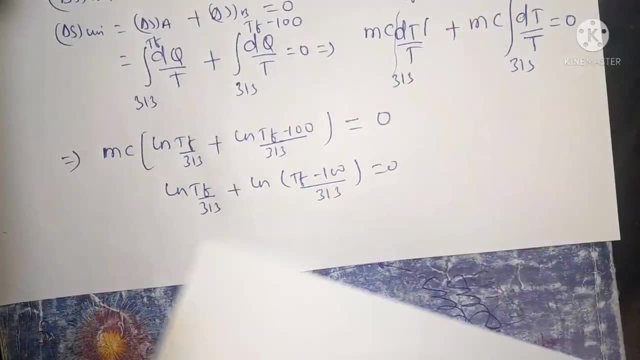 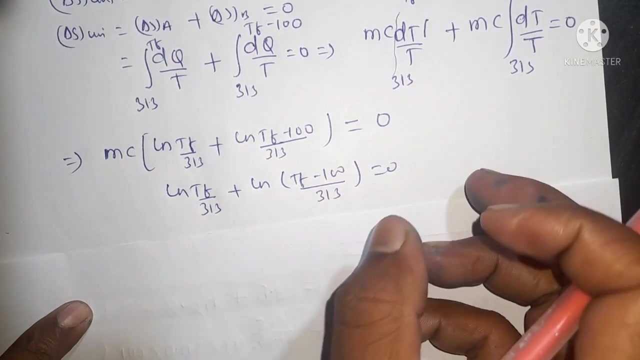 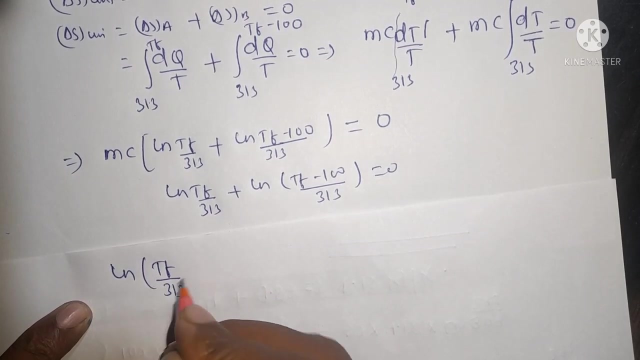 plus l and tf minus 100 by 313 into zero. equal to zero. ok, equal to zero. now what will happen? so you know the property of log when it is in: add you will multiply it. so your l and tf by 313 into tf minus 100. 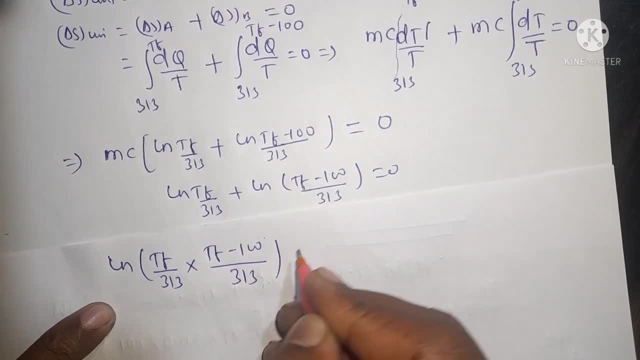 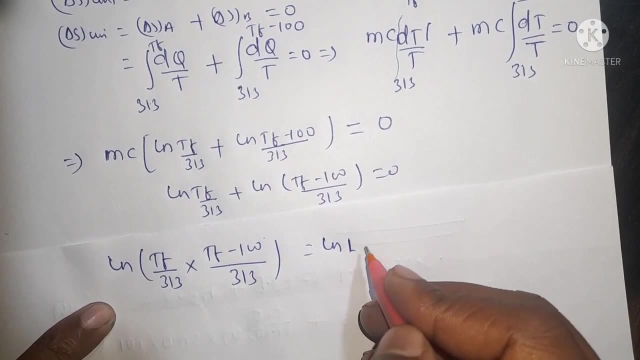 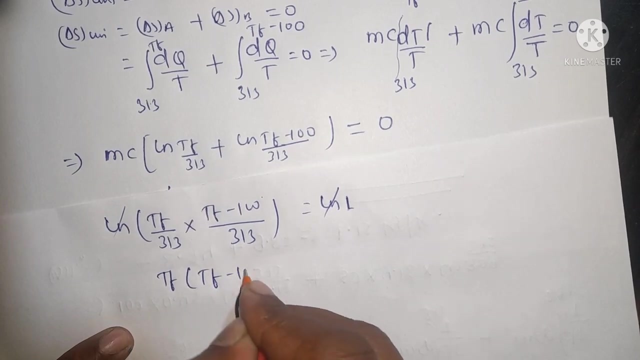 by 313 and zero, you can write ln, ln1. and why you can write ln1? because the value of ln1 is zero, so we can write ln1 instead of zero. then ln will be cancelled out. your tf tf into tf minus 100, equal to your square here. 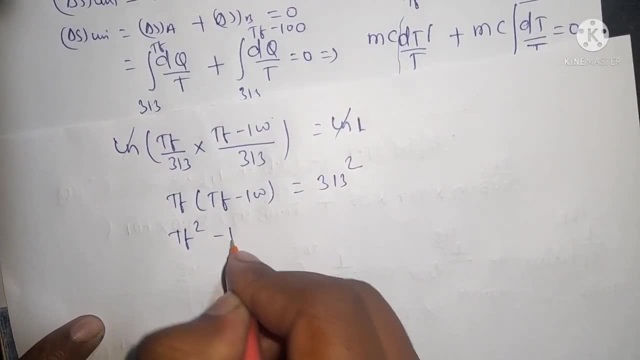 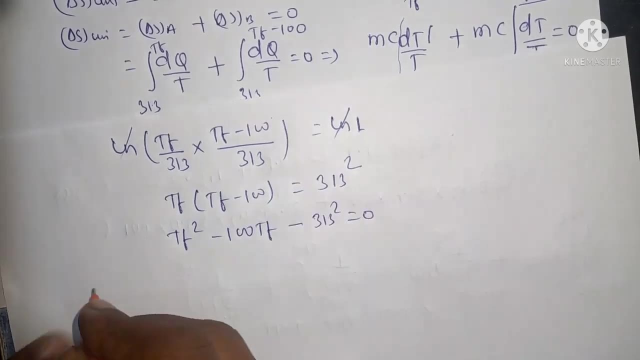 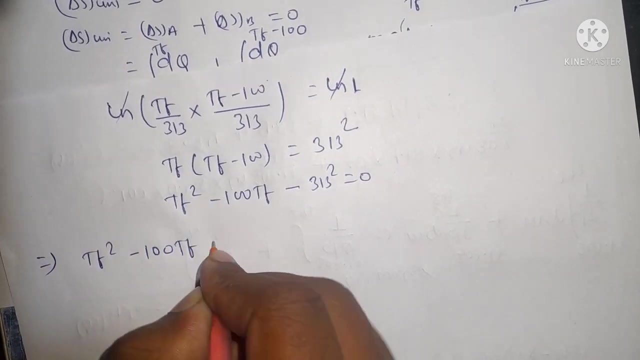 so now, tf square minus 100 tf, and when your plus will come here, minus will come here: 313 square, equal to zero. ok, now what you have to do: tf square minus 100 tf when square will be 9,7,9,6,9, equal to zero. 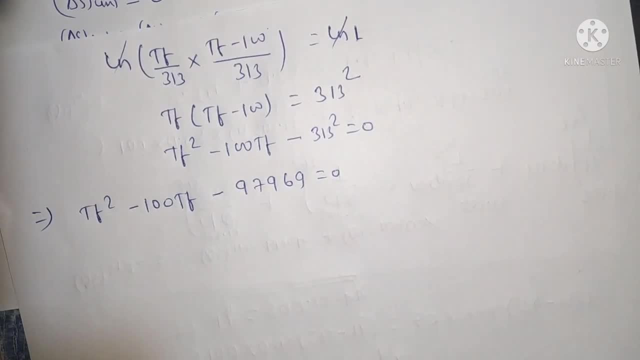 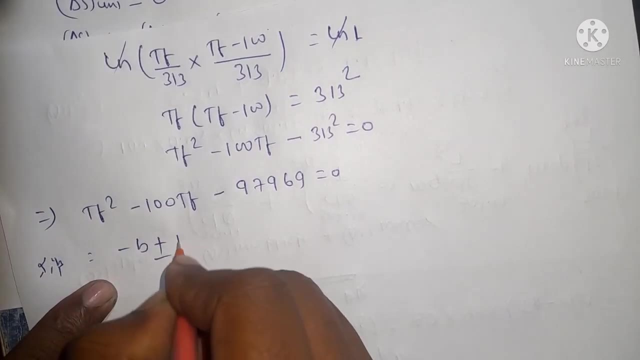 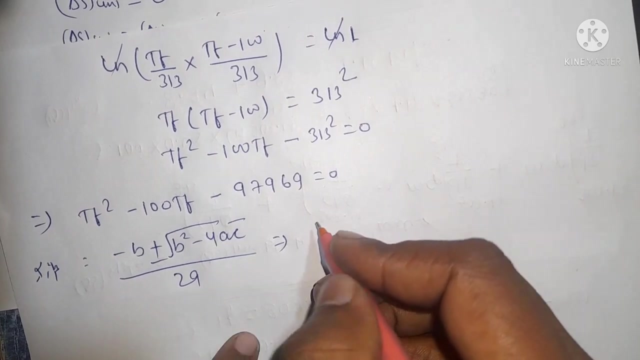 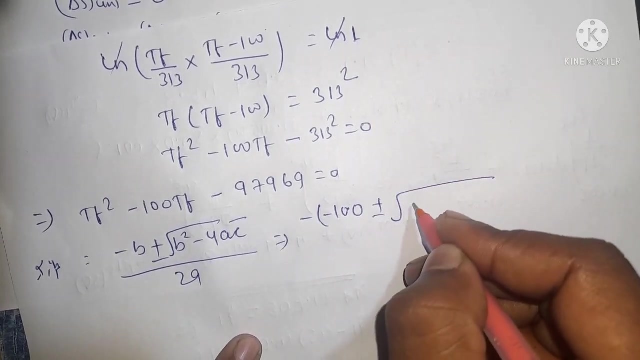 when we will take out its roots alpha and beta. alpha and beta means minus b plus minus root under b square minus 4ac by 2a. when we will put this value, minus b, equal to minus, into minus 100 plus minus b square minus 100 square. 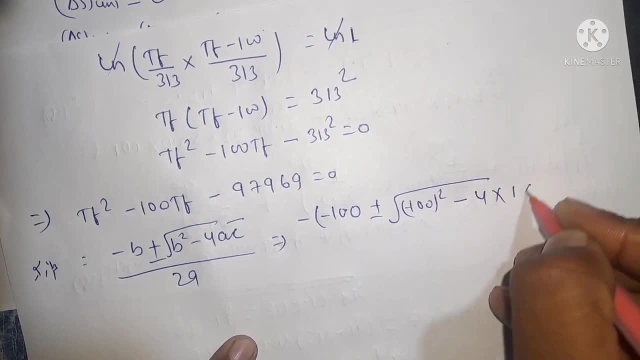 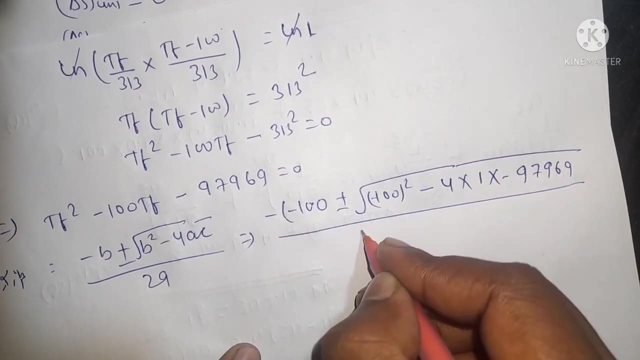 plus minus 4a, how much is 1 plus c? how much is 9,7,9,7,9,7, 7, 9,, 6, 9 And by 2a, 2 and a's value is 1. 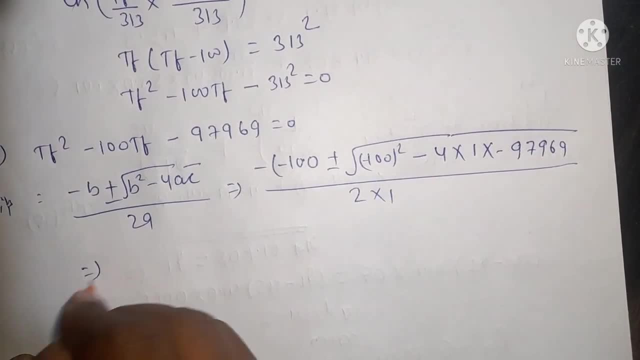 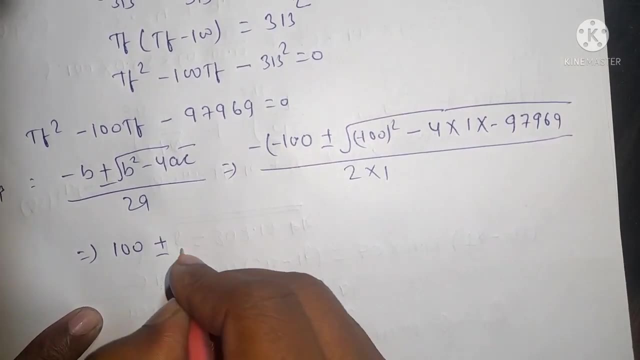 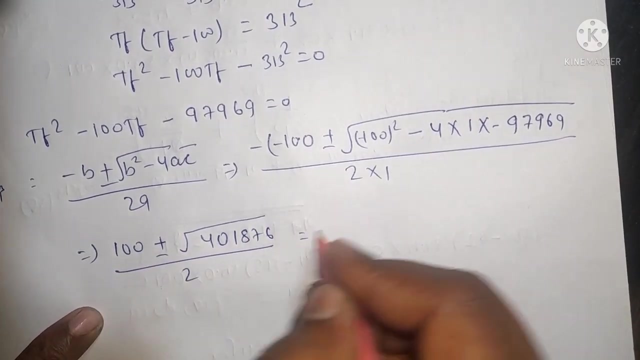 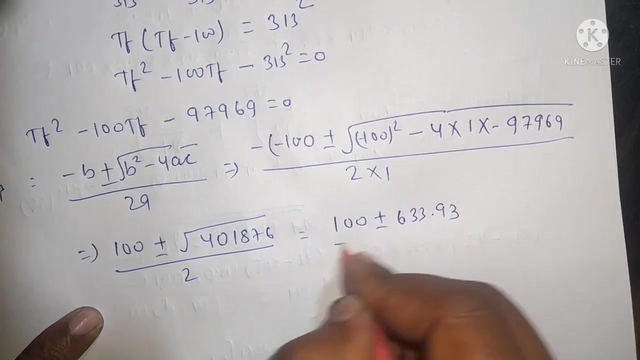 Ok, a's value is 1 When you solve it. How much will it be? 100, 100 plus minus minus plus Into 401876 By 2. When you solve it, 100 plus minus 633, 9,, 3 By 2 When it has alpha and beta. 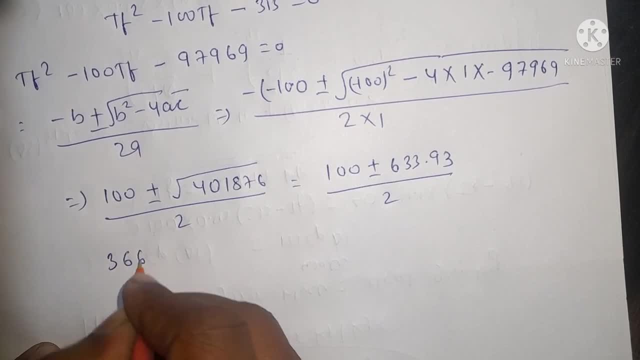 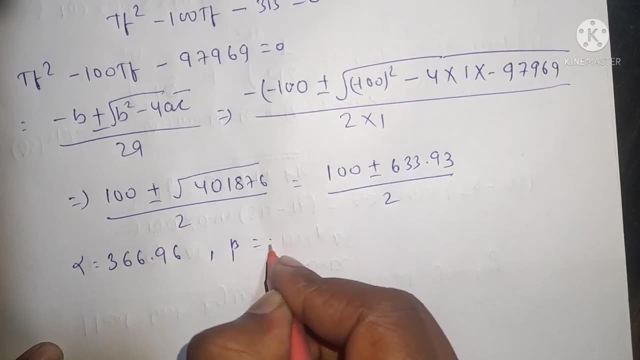 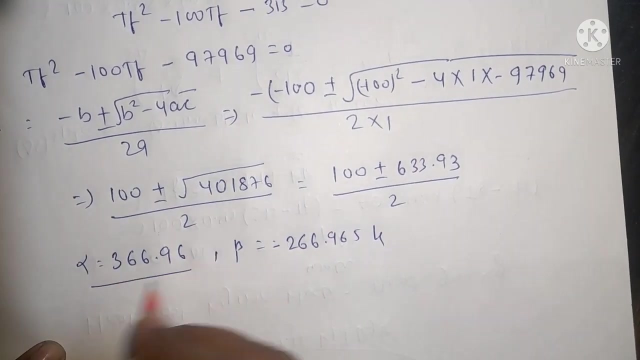 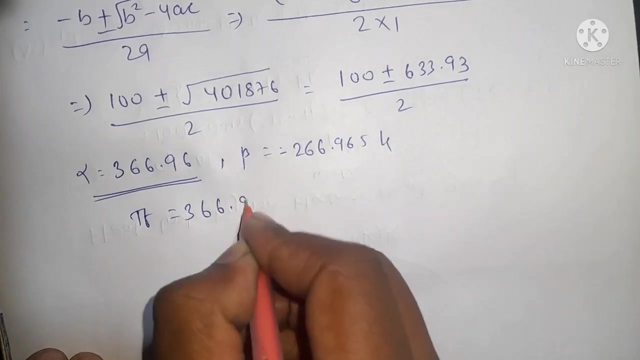 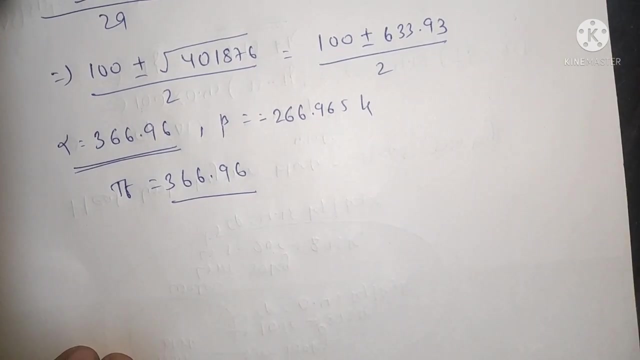 Two values. One will be 366.96 And second will be Alpha and beta Minus 266 965 Kelvin. Positive value: Tf value: 366: 6.96. Negative Positive: 366.96. So now see Now what to do. Find out the value of our tf. 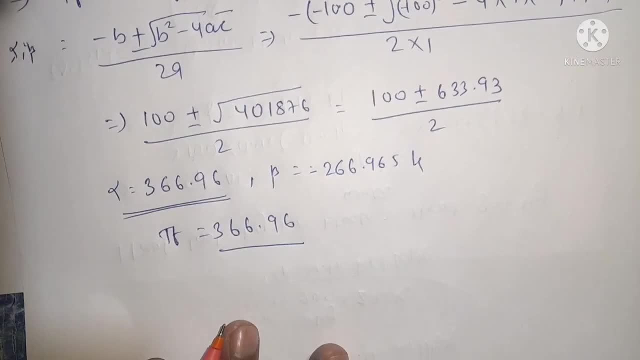 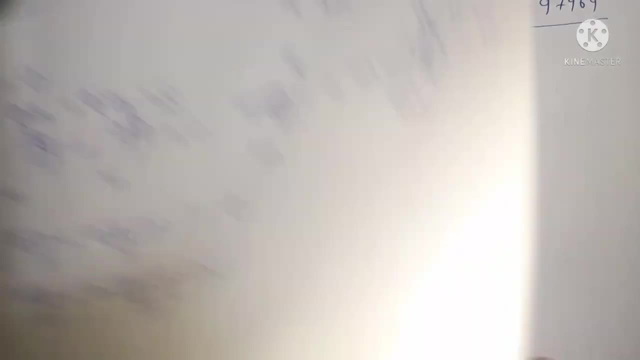 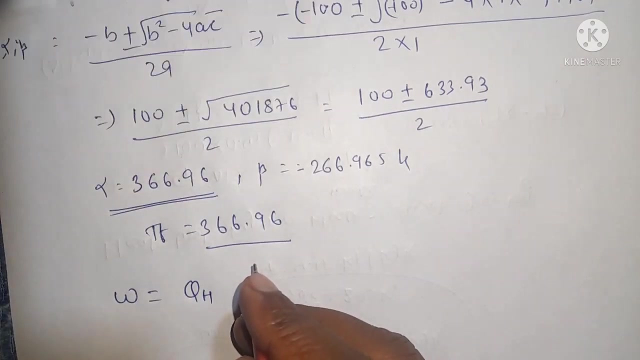 So our tf value is found. So what I have to do, I have to find out the work. So what is the formula of work? Work is qh. See Who is qh. So suppose you do qh And do ql So qh. So qh is qh. 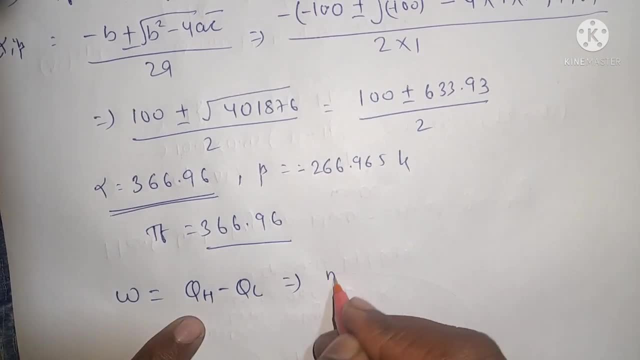 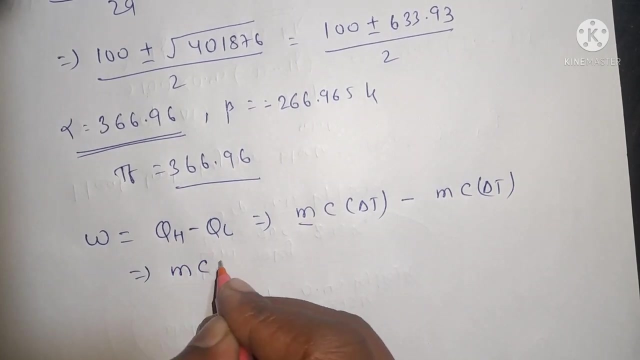 So qh minus ql. So what is the formula of qh mc into Delty? The minus of heat, Minus of mc Into delty Is okay, This is also delty. So now what to do? That the mass of both is same, So m And c. 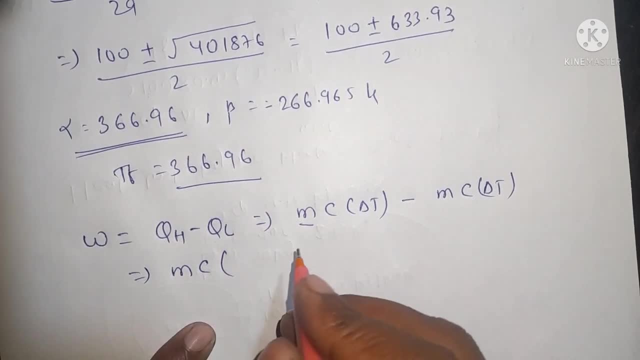 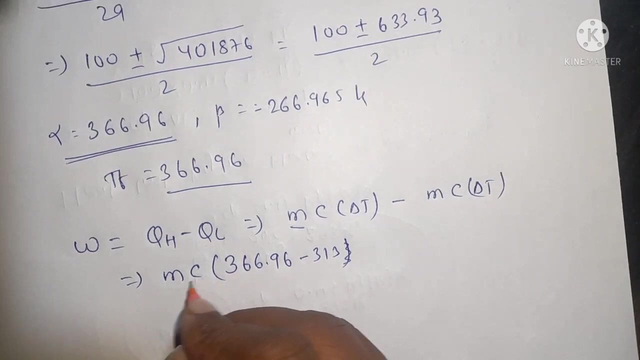 Out. Its temperature difference. Which is your higher temperature? What was the previous one? Your previous one Your higher temperature? Because here I mean by magnitude. So 366.96, 366.96, 96 minus 3, 13, 13, 13, 36 minus 13 mc. 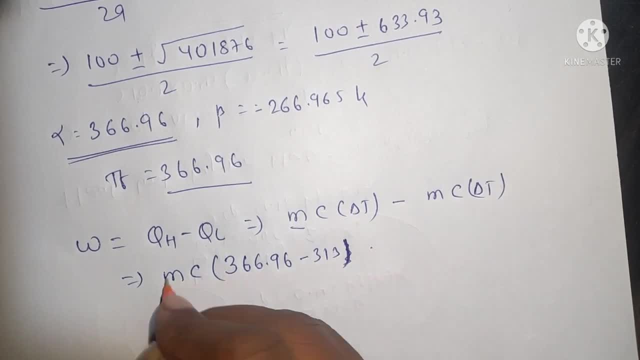 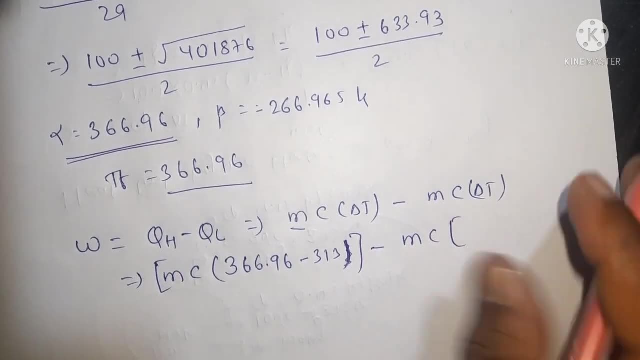 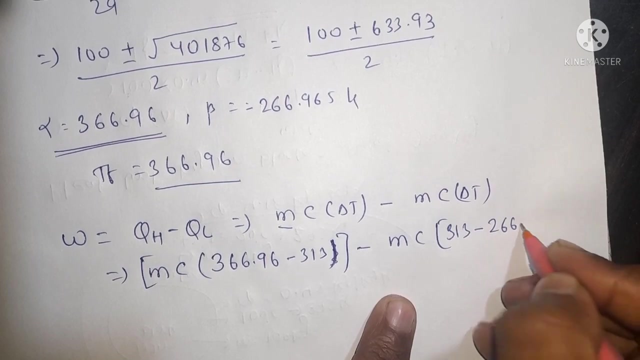 This is not a common. First take a common. This is your one, Done Here, Okay, And minus mc Into And its temperature difference Because Body was also low temperature. So what was your previous temperature? From 313 Because 266.96. What will happen here? See here What is the value of our body. 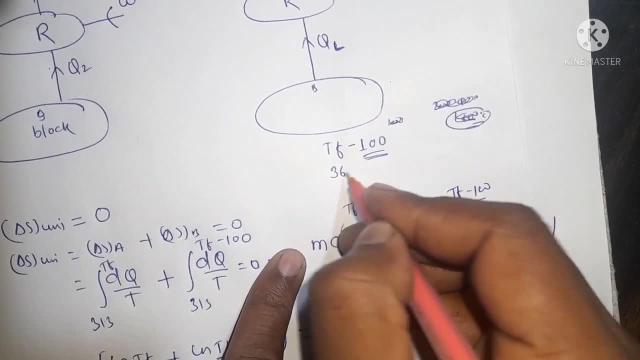 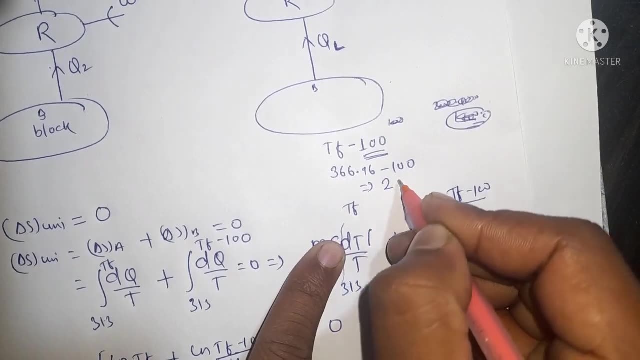 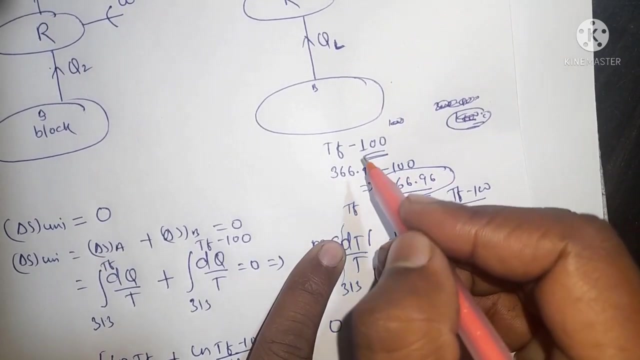 How much did the value of tf come Now? the value of tf is 366, 366.96 When we subtract 100 in this. So how much will we get? So 266.96? Is this much temperature or not? Because we always have to keep the temperature difference 100. 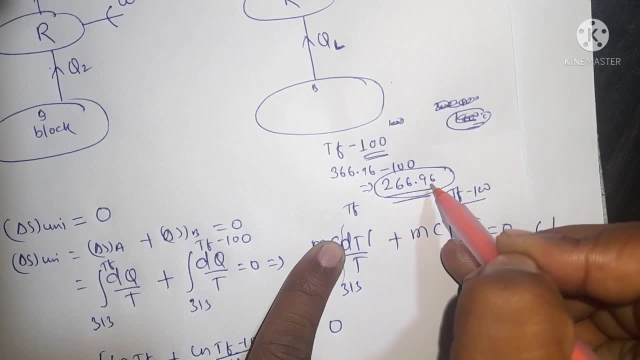 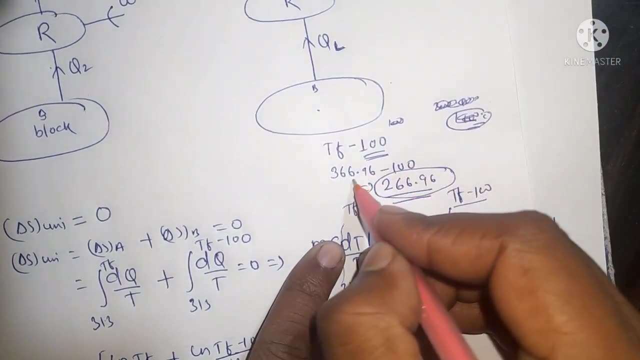 So how much will our tf be? 366.96, So our 266.96. Our b will be its temperature, Then the temperature difference between our system a and b will be It will be 100. Okay, So now see this much. So now we are doing mcp. 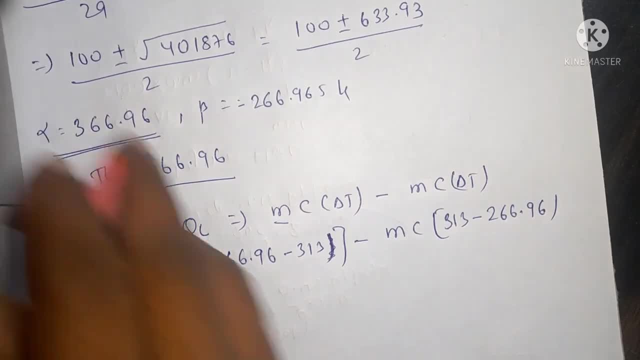 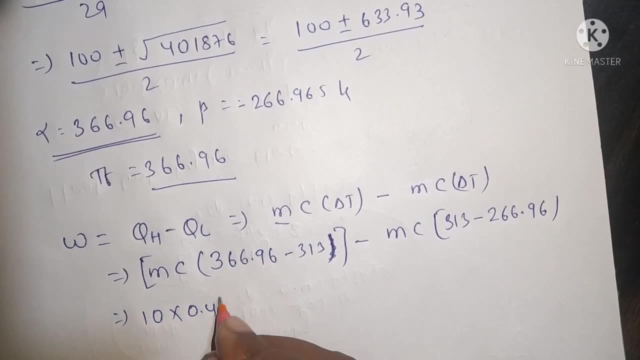 We are doing mc out, So the values of mc and q are the same. So how much mass have you given? The mass given to you is 10. Into specific heat, It is given to you 0.4. Take it out And see this: 366.96 minus 313. 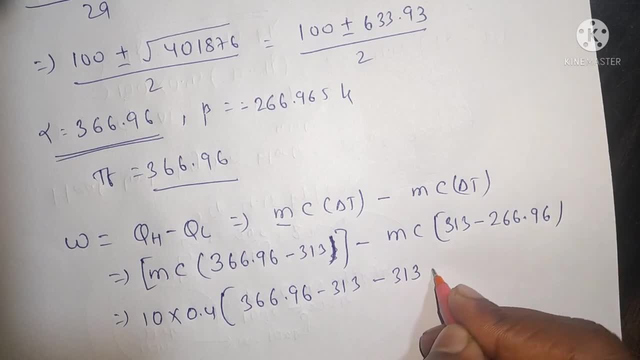 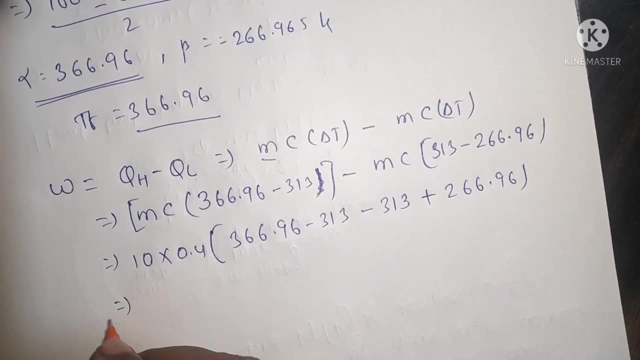 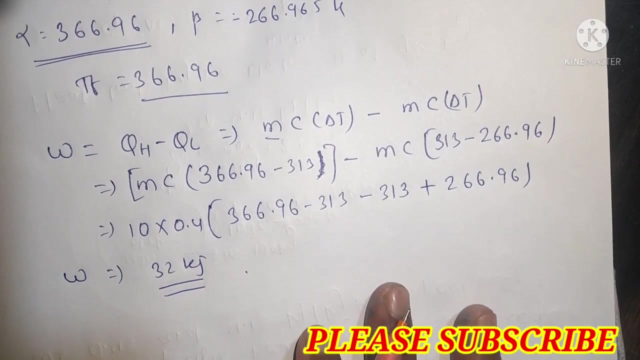 And your minus 313 And this will be plus 266.96. When you solve this, Then the value of your work will be. How much will it be? 32 kilojoules Will be.